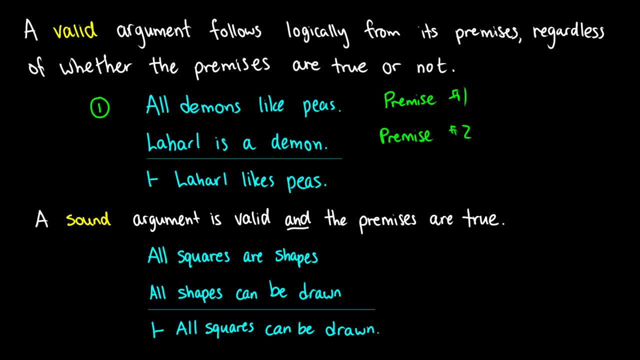 shouldn't have the s on the end there. So premise one, premise two, And we have a conclusion underneath the bar And we use this little symbol here. This is a symbol of a proof that tells us whether the argument is valid or not. So we can think of this argument as having 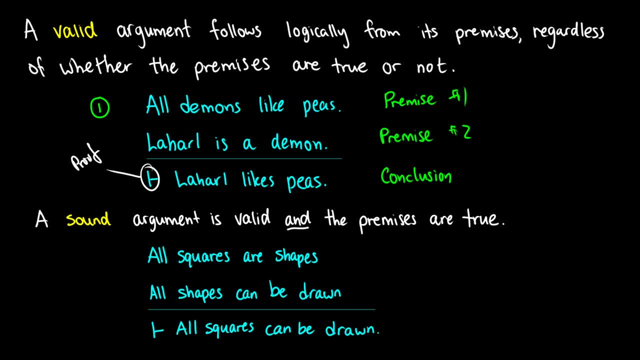 two premises. So this argument says: all demons like peas. Laharl is a demon, Therefore Laharl likes peas. So this is a valid argument because structurally the conclusion follows from the premises. But in this case we don't know if this first line is true. We don't know. 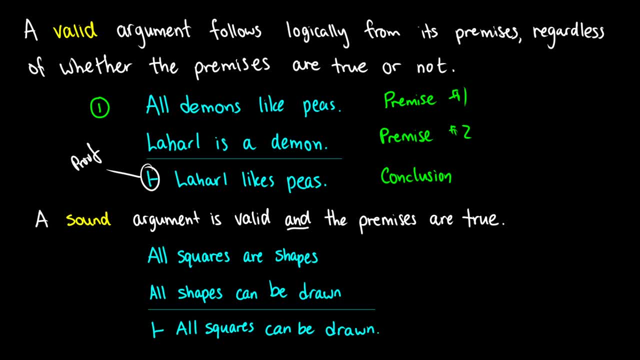 if the second line is true. So when we talk about arguments, valid arguments that have true premises, we call those premises. So this argument says: all demons, like peas Laharl is a demon. So that's when we know that the premise is true. So, for instance, in this argument, all squares. 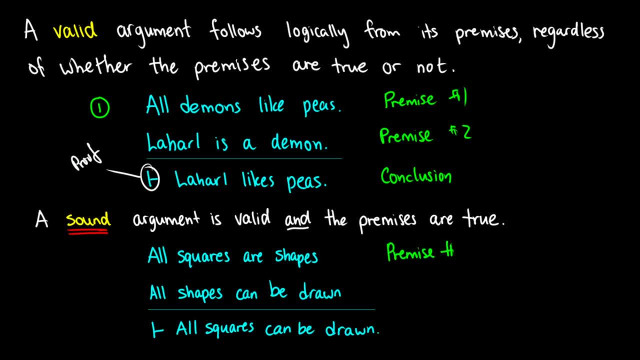 are shapes. Okay, this is premise number one. This is a true premise. All squares are, in fact, shapes. Premise number two: all shapes can be drawn. Okay, that is also true. If we scale them down small enough, we can draw any single shape in the world, provided it's two dimension. 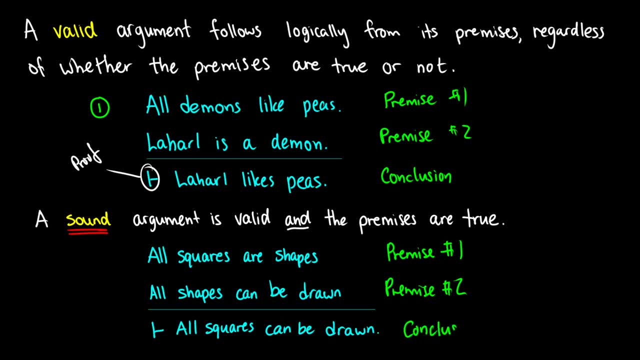 Therefore our conclusion all squares can be drawn. So it's valid because of the structure, We know that the premises entail the conclusion- And it's also sound because in this case our premises are true. Premise number one is true and premise 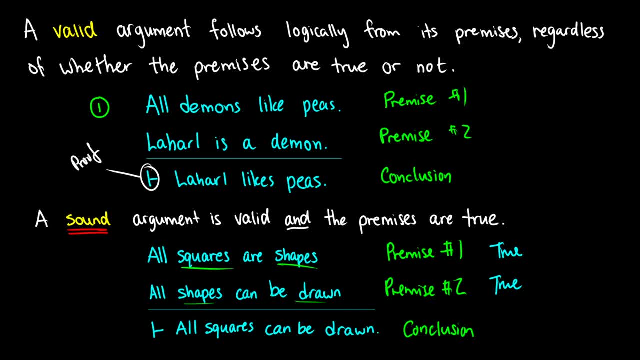 number two is true. So that's the difference between a sound and a valid argument. Now, in a logic course, we don't care too much about soundness, It's more so about just working with real things, So that way we can apply these to real things in the real world And then in the 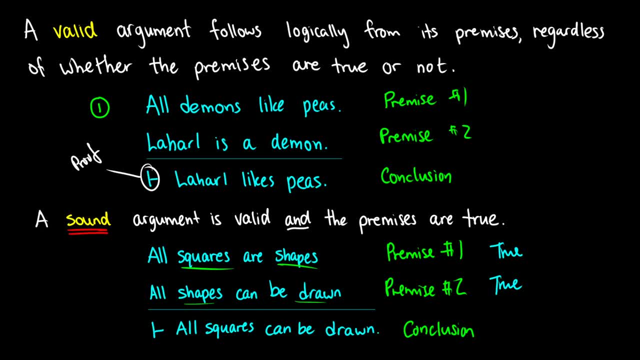 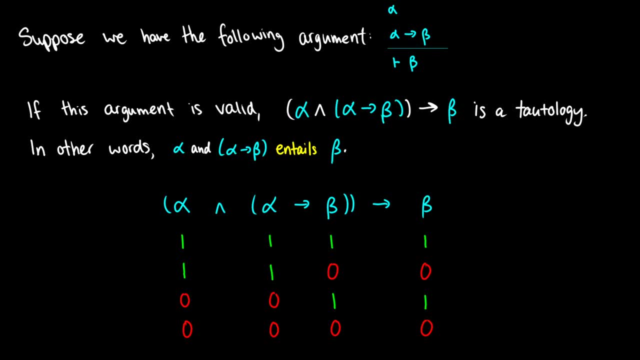 real world we care about soundness, But mathematically we don't care too much about. So let's suppose we have the following argument: two premises and a conclusion. We have alpha, that's premise number one. We have alpha arrow beta, that's premise number two. 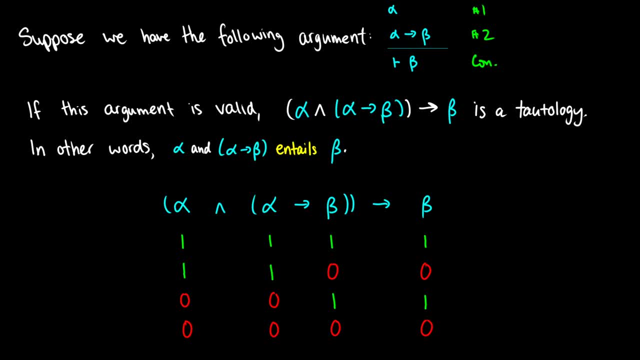 And then we have our conclusion: beta. So if this argument is valid, this means that if we have alpha and we have alpha arrow beta, we get beta. So we can think of this as saying that alpha and alpha arrow beta, arrow beta is a tautology. What that means is that if the premises are true, so if 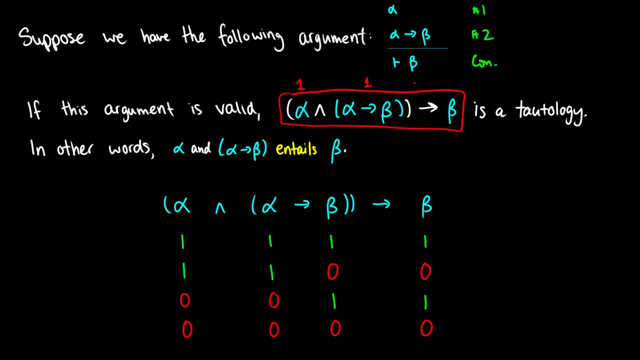 alpha is true and alpha arrow, beta is true, then it must be the case that beta is true. If beta is false, in that case it is not valid. If our premises are true, then our conclusion should also be true. So one arrow, one should happen, or zero. arrow one or zero. 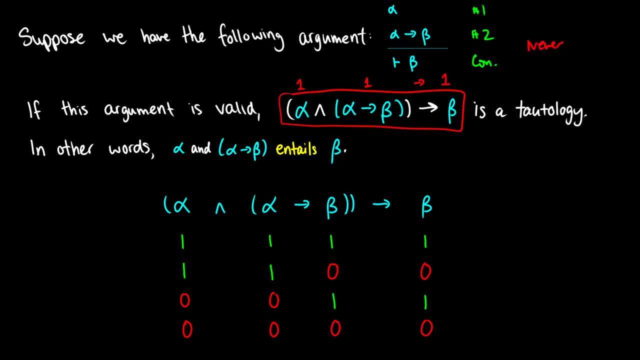 arrow zero. we should never, never, have one arrow zero. Another way of saying this is that alpha and alpha arrow beta entails beta. this is another word for that. So we need to check with our truth table to see if this is a valid argument. So I'm going to clear this up a little bit, just so that. 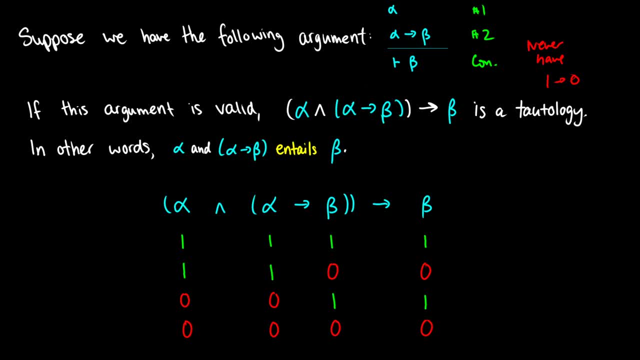 way, it's not too crowded. But we need to show that this argument is a tautology. So this row right here, or this column with our conditional- that's, our main connective- should be a tautology if this is valid. So let's do our truth. 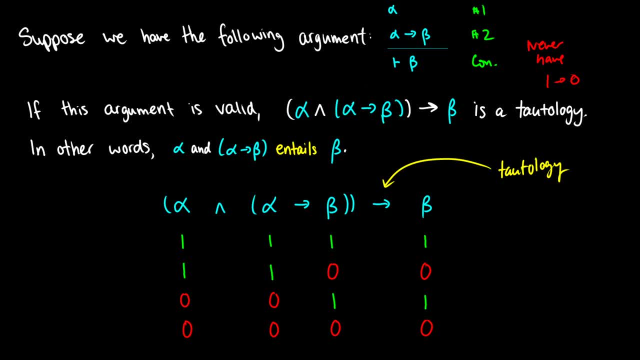 tables And I will go through this a little bit quickly because we've done these so many times already: Alpha arrow beta. this will be true in rows one, three and four, because we have one arrow, one zero. arrow one zero, arrow zero. it'll be false in row two: one arrows zero, it's the. 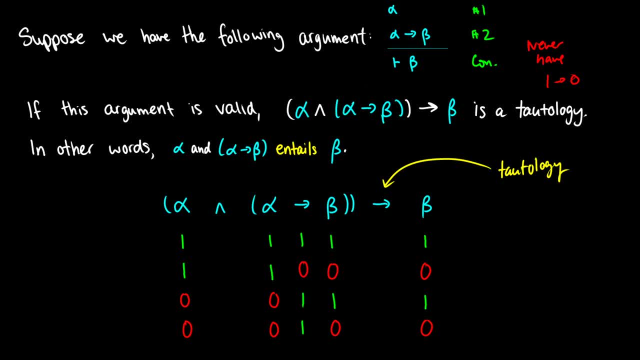 only time it's false With the. and here we're taking information from alpha, information from alpha arrow beta, so those both have to be true. So one one in the first row, that's true. One zero in the second row, that's. 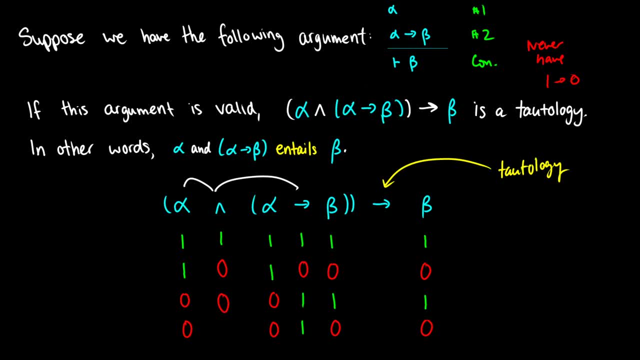 false Zero. one in the third row- that's false. Zero one in the fourth row- that is false. Okay, so we just have one more step to go. we just have to do the arrow here, And the arrow is going to take. 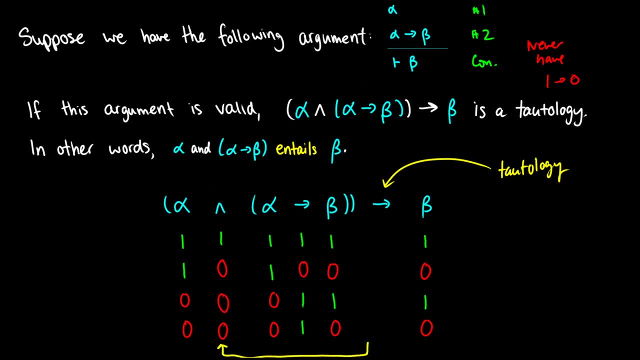 information from this column. So the and for alpha and alpha arrow beta And it's going to take information from beta. So it's only false if we have one arrow zero. So the first column or the first row, we have one. 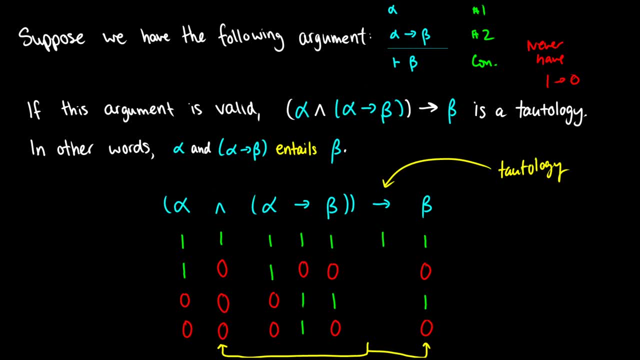 arrow one, that's true. Second row: zero- arrow zero, that's true. Third row: zero- arrow one, that's true. Fourth row: zero- arrow zero, that's true. Great, We're finished here. We have found that the entire wellformed 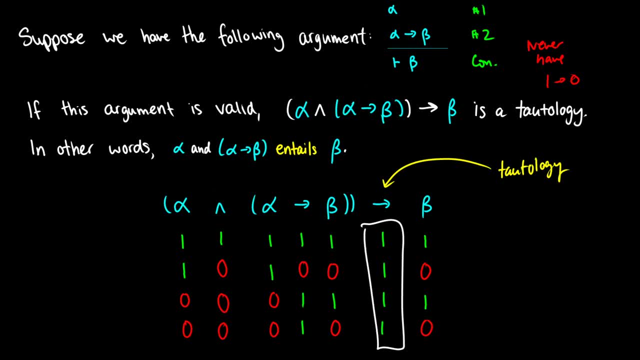 formula here in this column is a tautology. It's all ones. Therefore, we know that this is a valid argument. We know that when we have premise number one and we have premise number two, what we get is the conclusion. So, no matter what the assignment for alpha and alpha arrow beta is, we get beta out. 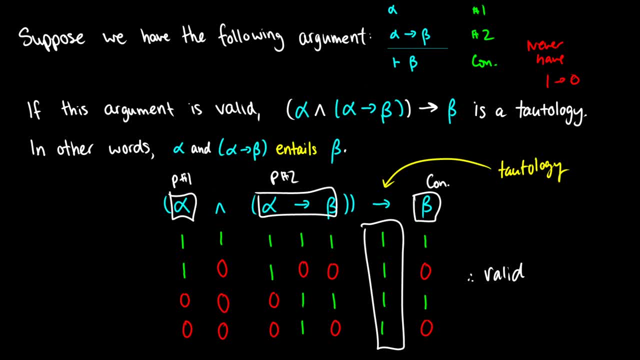 of it. So it's a valid argument because we have those two entailing the third. and, as a reminder, how did we get here? Well, we took a look at our argument at the top. So we take our premises, we put ands between all the premises, we take our conclusion, we put an arrow before it, Don't worry. 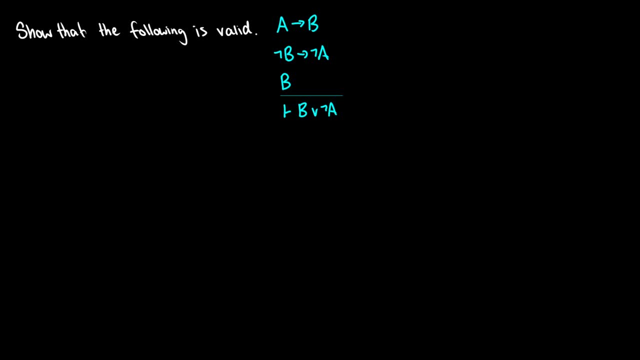 we have a another example here. So let's show that the following is valid: a arrow b, not b. arrow not a b. therefore we have a tautology, So we know that this is a valid argument because we have those two entailing b or not a. Okay, so I'm going to set this up, So what I need to do and I'll put on. 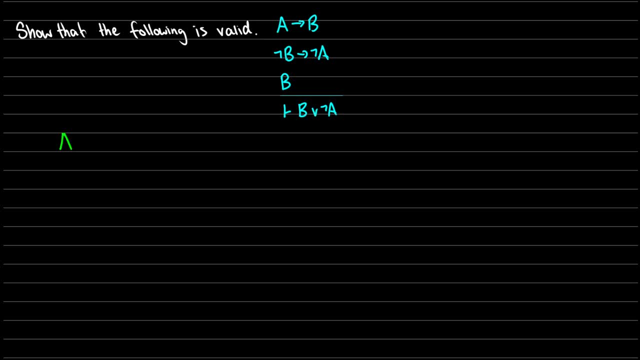 some lines for this, so it looks a little bit nicer. We have alpha or, sorry, we have a arrow b. that's premise number one. We take an and we add our next one, not b arrow, not a. Okay, we're going to take an and we'll add our next premise b. Okay, now we're going to put an arrow before our. 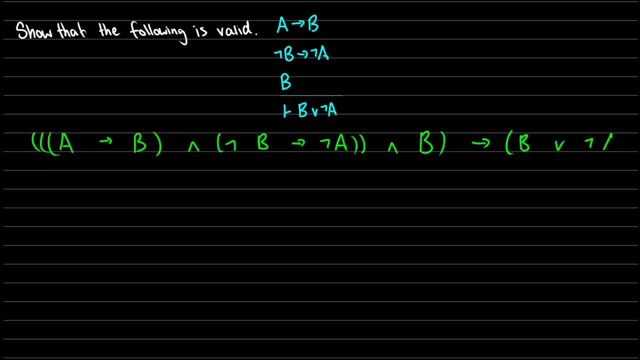 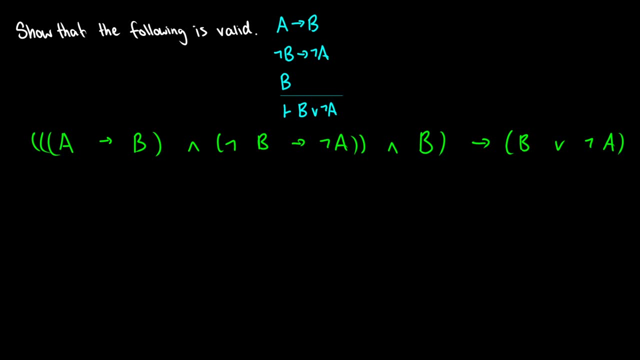 conclusion, which is b or not a. Okay, so this is what we have to show is a tautology, and we need to show this on our main connective here. So this column under the arrow should be a tautology. Now, what I'm going to do is: 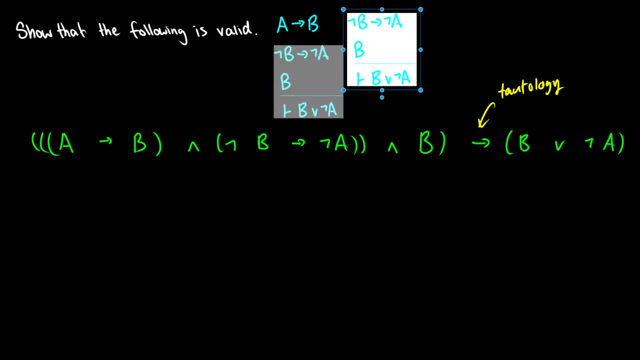 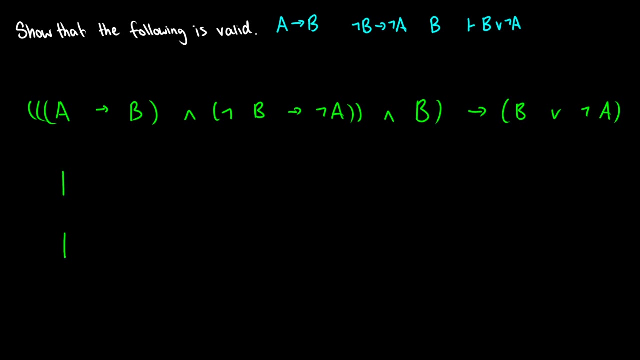 I'm going to, I'm going to move over this argument a little bit, just so that way we have some more space to work with this truth table. So let's move this up a little bit and let's start our truth table. So a will be 1 1 0 0, b will be 1 0, 1 0.. 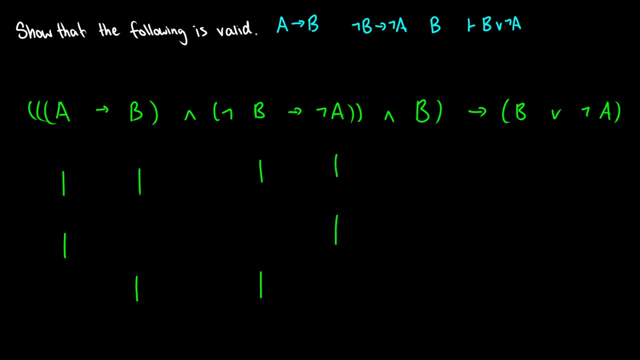 So I'm going to set up the a's and the b's right now, and hopefully these all align nicely. Okay, now let's fill in our zeros for our truth table. Okay, so we have our truth table set up. Now we're going to have to do this piece by piece, So we'll start with a arrow b. This is our simple 1: 0, 1, 1 truth table that we did on the previous example. 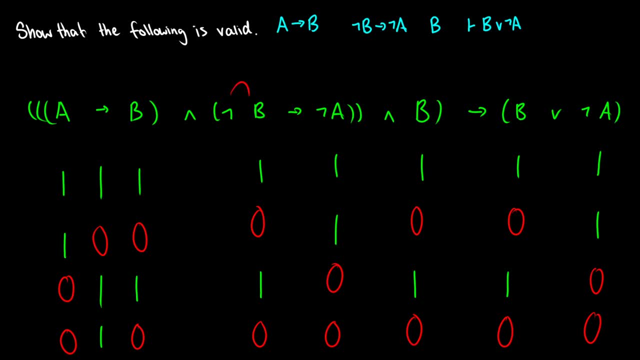 Not b. this will flip the values of b, So in this case, so 1 0 1 0 will become 0 1 0 1.. Okay, it'll be the same thing with not a here, So 1 1 0 0 will become 0 0 1 1.. 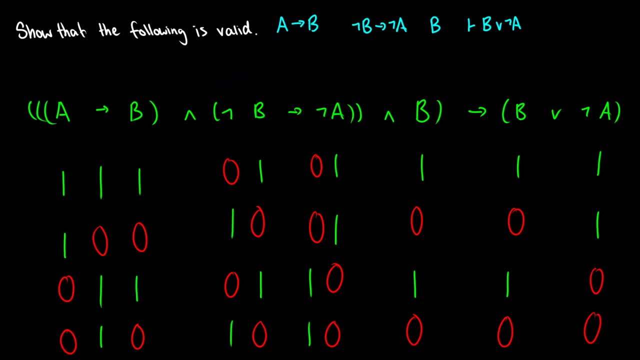 Okay, is there any more negations we can do? in our truth, table Yes, not a, over on the right here. So 1 1 0 0 will become 0 0 1 1.. Okay, so we've done our negations. What do we have left? Well, let's do not b arrow, not a. 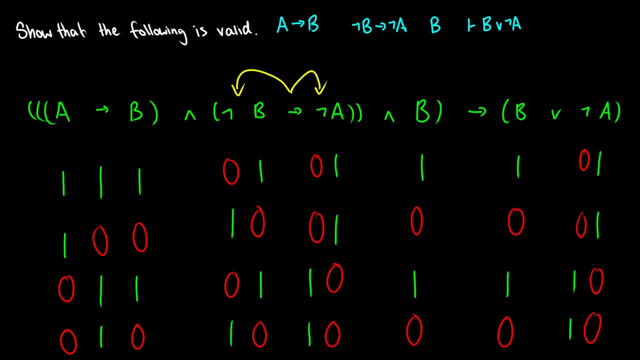 So we're going to be looking at the not columns here and we'll be looking for 1 arrow 0 to make that false. In the first row, we have 0 arrow 0- that's true. Second row: we have 1 arrow 0- that is false. Third row: we have 0 arrow 1- that's true. and fourth row, we have 1 arrow 1- that is true. 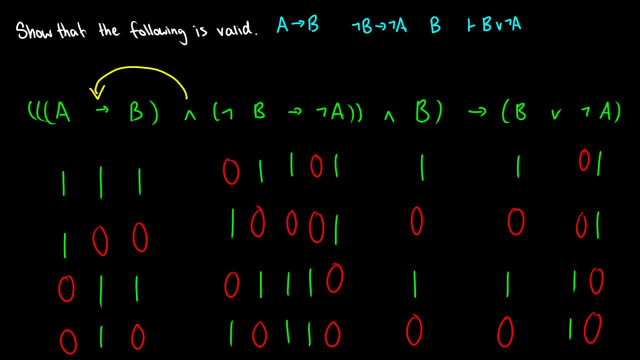 Okay, let's now do and. So and is going to take information from our a arrow b, and it's going to take information from our not b arrow, not a, So I'll just put little boxes around here. So both of those have to be true for the conjunction to be true. So we have 1 and 1 and 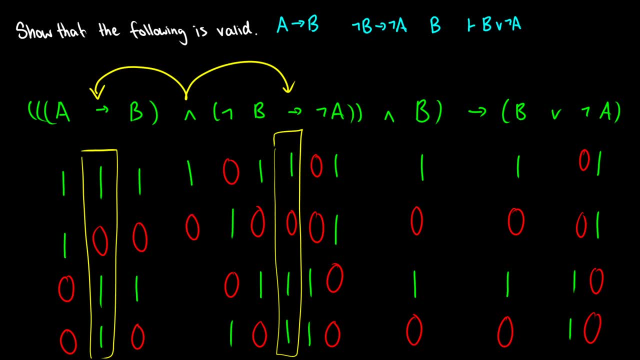 first row, that's true. Second row: we have 0, 0,, so that's going to give us 0.. And in the third and fourth rows we have 1 and 1, that gives us some 1s here. Okay, so that 1 is now done. 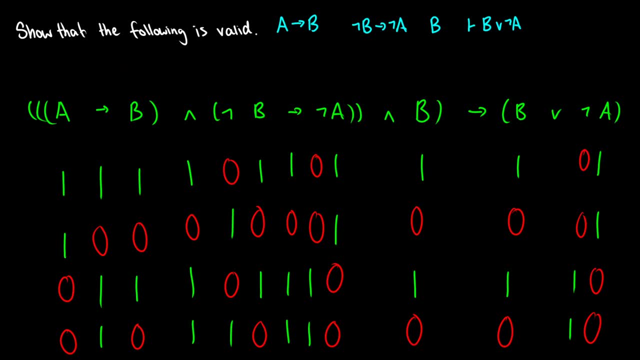 What do we have next? Oh, we have this AND right here. So this gets information from B and it gets information from our AND column here. So remember, it's going to be true when both of those are true. So I need to make this box a little bit thinner so I can fit that there. 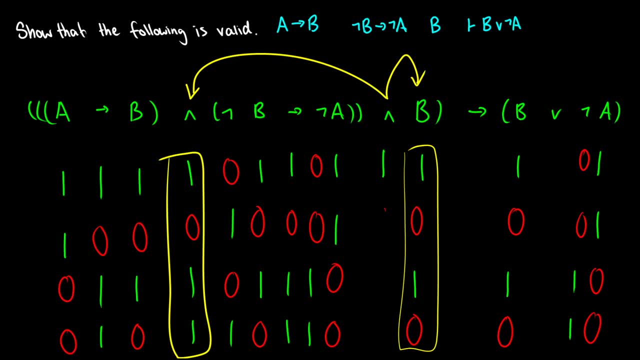 So we have 1 and 1 in the first row, 0 and 0 in the second row, 1 and 1 in the third row and 1 and 0 in the fourth row. That gives us a 1, 0,, 1, 0.. 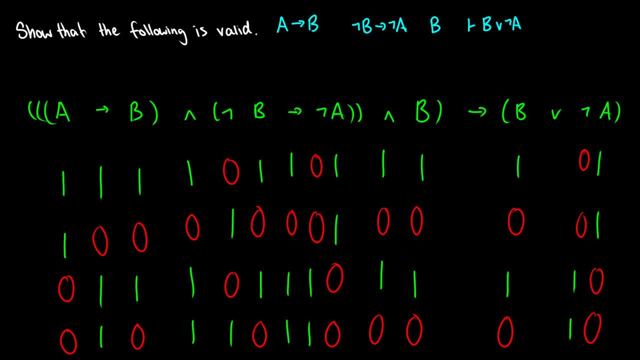 Okay, now we have to do B or not A. So B or not A. this is taking information from B, information from not, And just one of those things has to be true. So we have 1 or 0 in the first row, that's true. 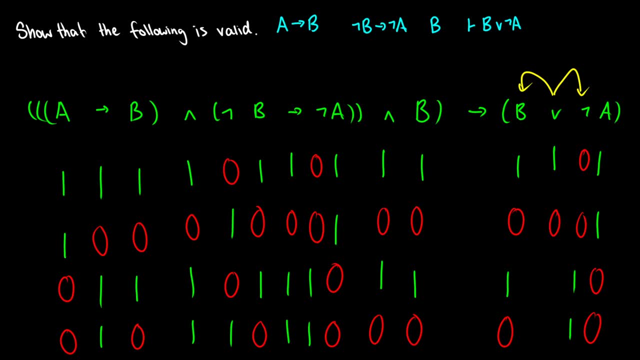 0 or 0 in the second row. that's false. Third row is 1 or 1, that's true. And fourth row is 0 or 1, so that's true. Okay, our last thing. This is the final thing we have to show. 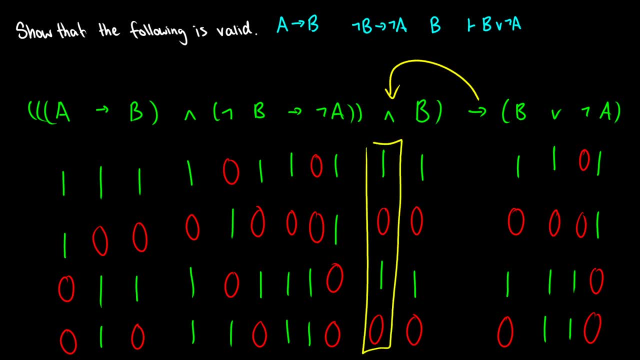 We take information from this AND here, because this represents the entirety of the antecedent, We get information from the OR. here, this gives us the entirety of the consequent, And we're just looking to make sure we do the same thing here. 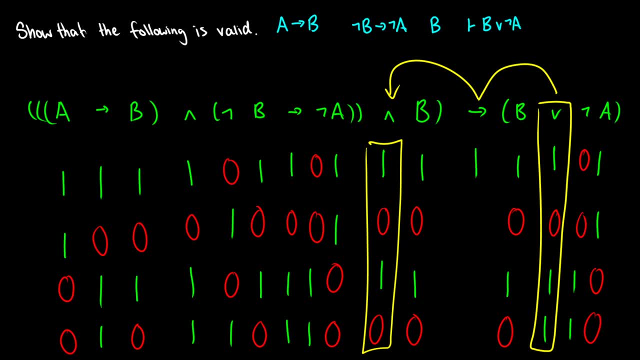 Because we do not have a 1 arrow 0.. So: 1 arrow 1, true. 0 arrow 0, true. 1 arrow 1, true. 0 arrow 1, true. Okay, perfect, We're now done. 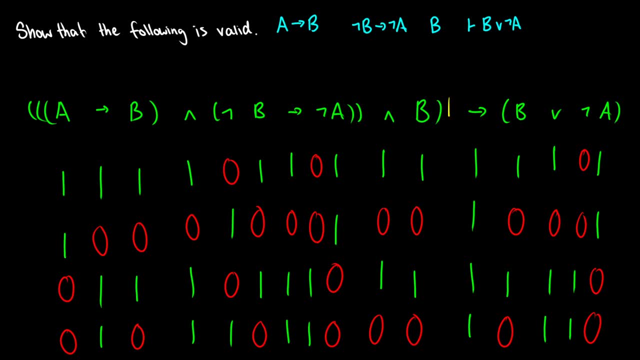 And what have we shown? We've shown that in this column that represents the entire truth table, we have a tautology And because we have a tautology, we know that the argument is valid if we have premise number 1, premise number 2,. 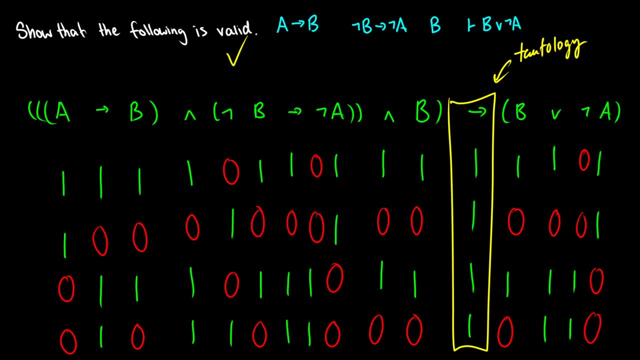 premise number three: we have to get the conclusion. So if we have one, one one, we have to get one. There is no way for us, using this truth table, to do one arrow zero. That is impossible. Therefore, this is valid. So that's how you prove validity using a truth table. We'll learn how to do it.